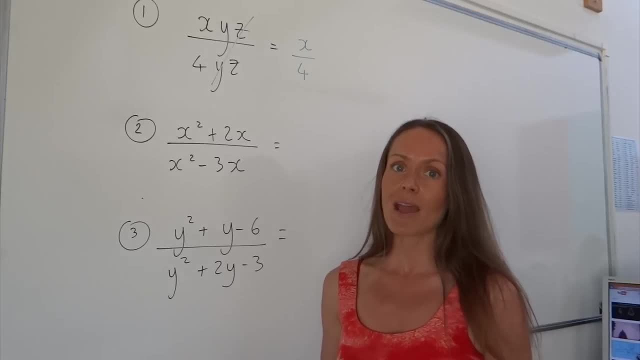 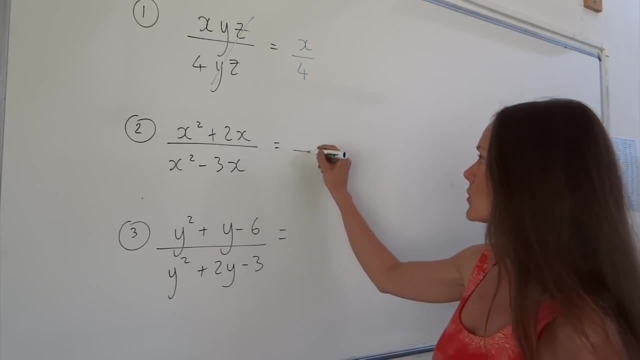 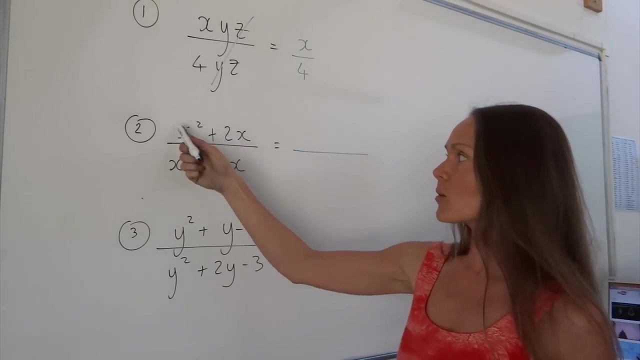 So if you've forgotten how to factorise, I really do recommend that you revise, Otherwise you're really going to struggle with these questions. So let's have a go at number two. This type of expression here is factorised into single brackets, And the highest common factor in these two terms here is just X. So to work, 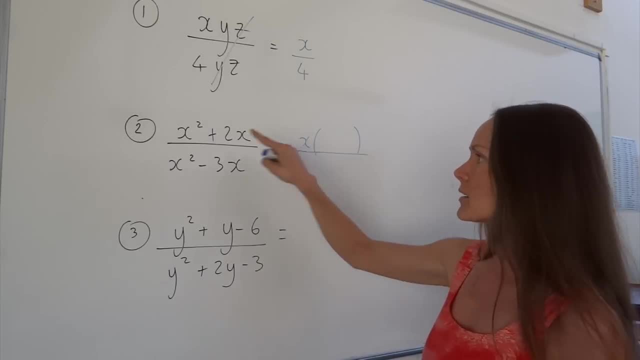 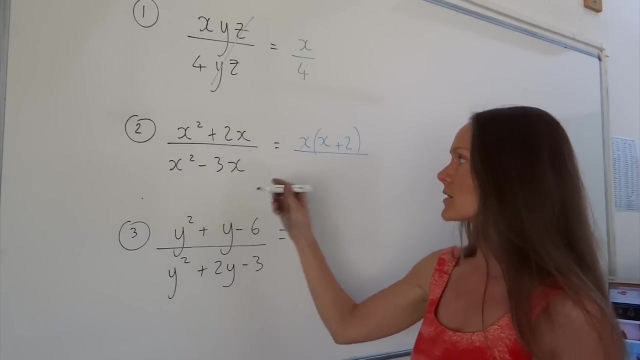 out what goes inside the brackets: X times something gives me X. squared Something must be X, And X times something gives me positive 2X. Well, that's just positive 2.. So I factorise the numerator. Now I'm going to do the same thing underneath, So I take out my highest common factor Again. 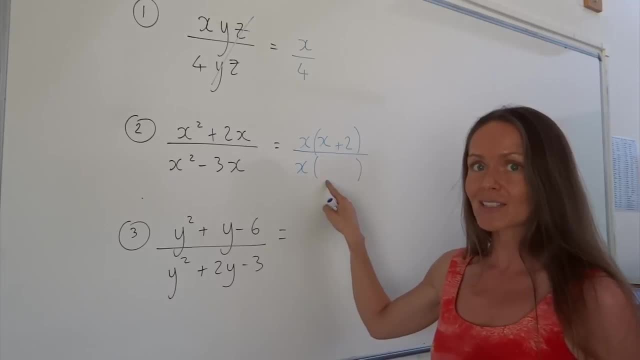 it's just X. And then, what do you multiply X by to get back to X squared, Just X. And what do you multiply X by to get back to negative 3X, Just negative 3.. Now I can see something that cancels. I've got X divided by X, which is just 1. So I can cross those out, And so 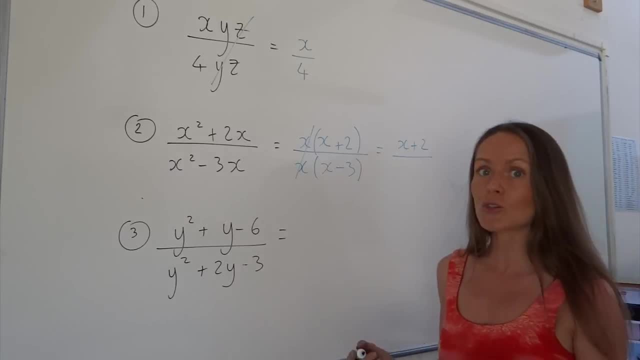 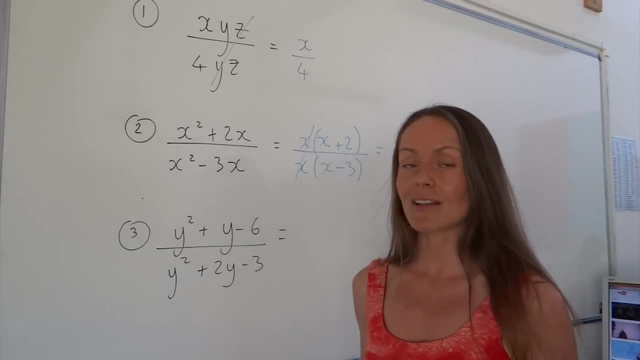 I'm left with my simplified fraction X plus 2 over X squared. So I've got X divided by X minus 3.. And that's done. All right on to number three. Now, this time when I'm factorising, I need a set of double. 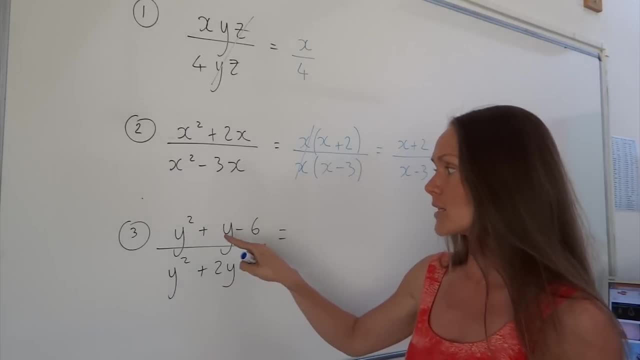 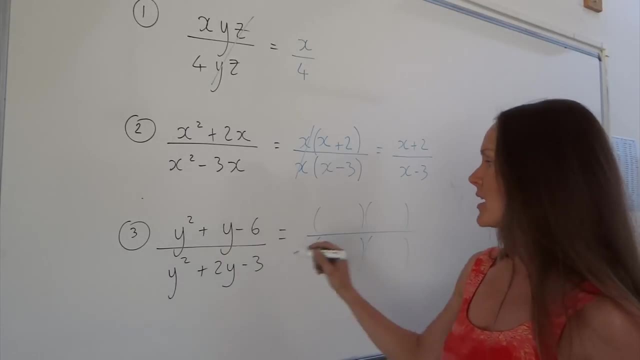 brackets on the top and also underneath, because it's Y squared, Y and a number. So I'm drawing those double brackets Now to get the Y squared. I'm going to fill in the Y values, because Y times Y is Y squared. Now remember, these two numbers that I fill in here must multiply. 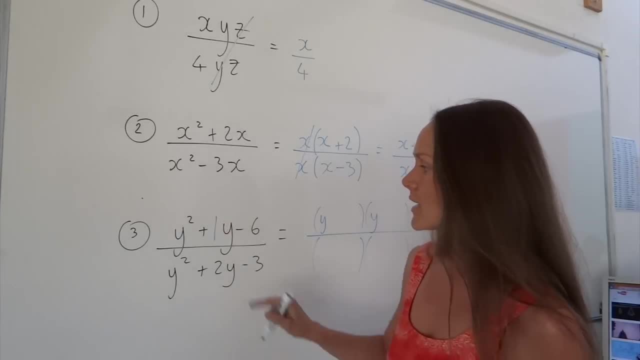 to give negative 6.. And they add up to negative 6.. So I'm going to add up to negative 6.. And the first two numbers that I've got are the Y and the Y squared, because they add up to give negative 6.. And then the second two numbers that I've got, I'll clean them up. 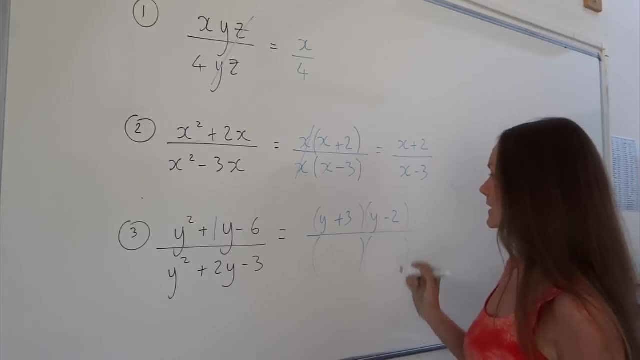 in the y-axis. And then they add up to give negative 6. And then I'm going to add up to give positive 1. So they must be positive 3 and negative 2, because 3 times minus 2. 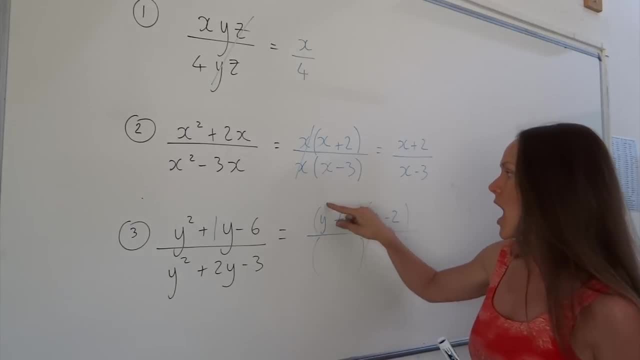 gives me the minus 6.. And then I've got a 3Y and a minus 2Y. that simplify to give me 1Y. Now for underneath Again, I'm going to just pop in those Y values there to get. 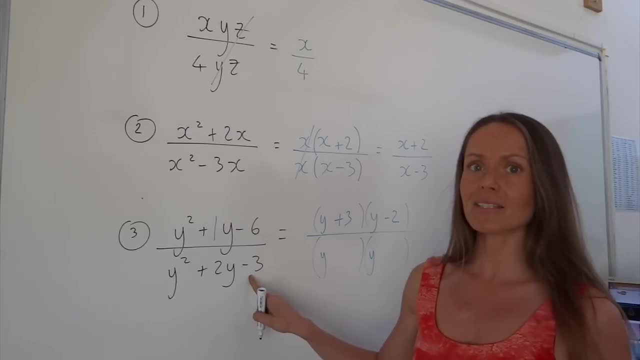 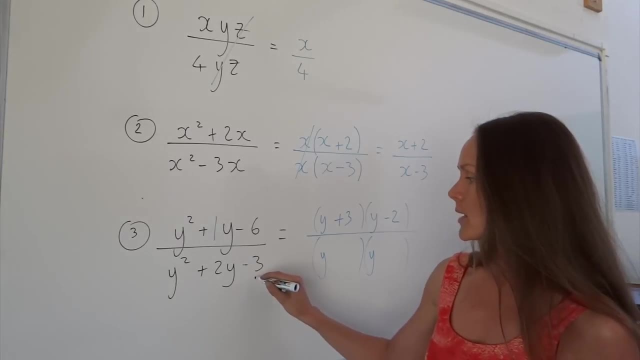 the Y squared And these two numbers multiply to give negative 3, and they must add to give 2.. Well, factors that multiply to give negative 3 could be 1 times negative 3 or negative 1 times 3.. They're my only options. 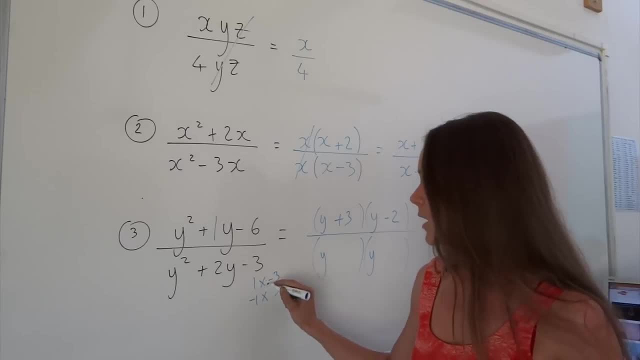 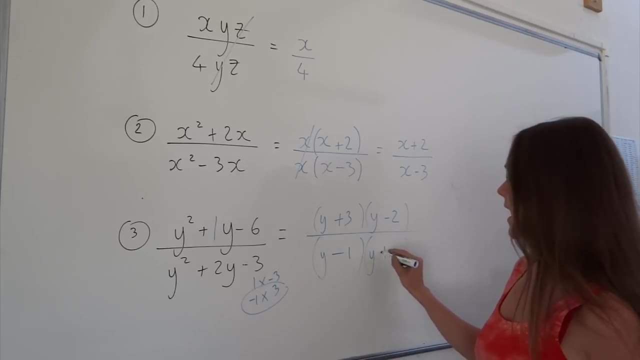 And the pair that add to give positive 2 are the bottom pair just there. So I need to fill in the values negative 1 and positive 3.. And it doesn't matter on the order, as long as the 1 is negative and the 3 is positive. 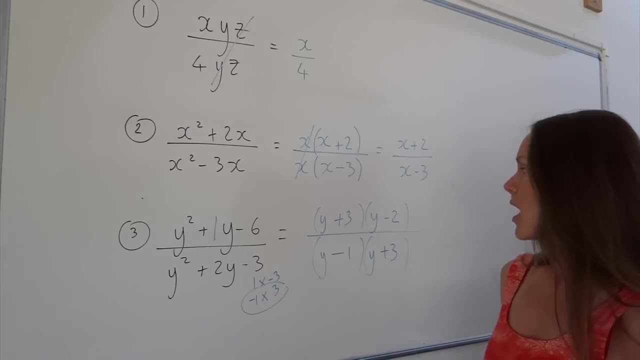 So hopefully now you can see what's going to cancel. I can see a bracket on the top that's the same as underneath. So y plus 3 divided by y plus 3 is 1.. So I'm just left with y minus 2 as the numerator and y minus 1 as the denominator. 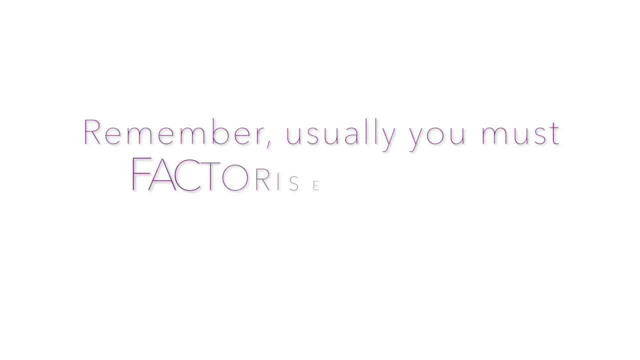 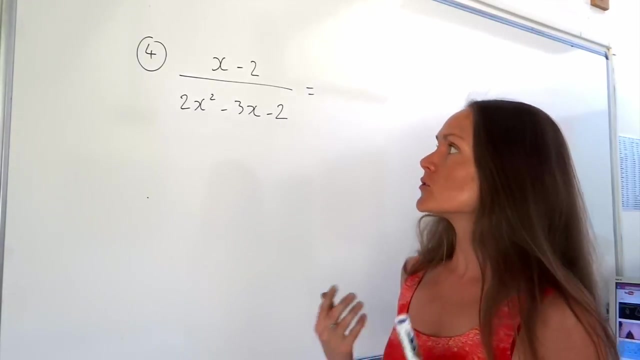 OK, on to the final question. OK, so here's my final simulation Simplifying fraction question, And I'm going to do the same thing before I'm going to look to see if I can factorise. Well, the numerator. I can't do anything with that. 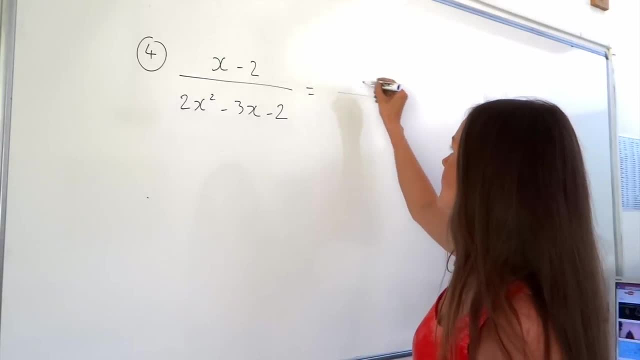 There's nothing that's common, So I'm just going to leave that as it is. The 1 underneath x squared x in the number. I know that goes into double brackets, OK, but it's a bit awkward when there's a number in front of the x squared. 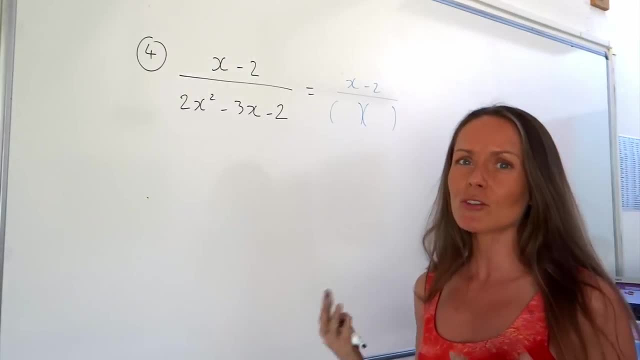 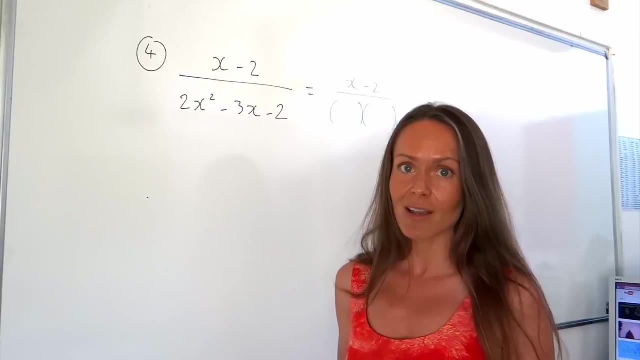 So I mean I could guess what goes in the brackets, but I don't really like to guess, So I'm going to use my method called PATH P-A-F. You might have seen it in one of my factorising videos. 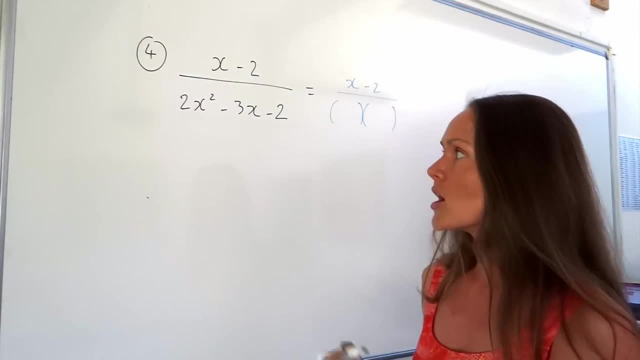 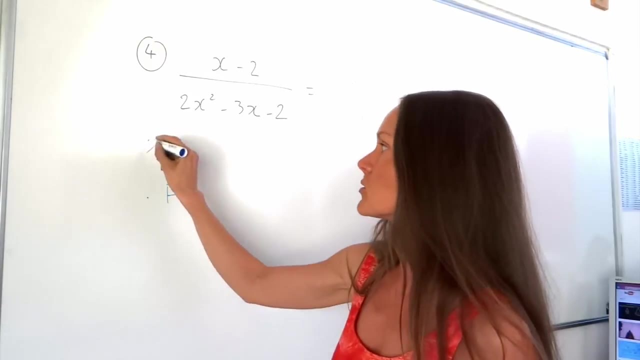 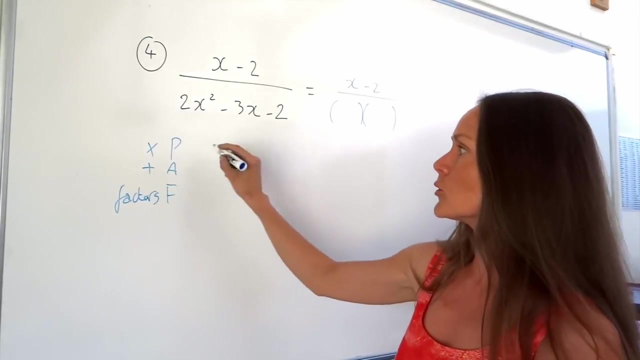 to work out what numbers go inside these double brackets. Remember when we've got PATH: P stands for product, A stands for addition and F stands for factors. So the product is just multiplying 2 by minus 2.. And the addition is this number, here the coefficient. 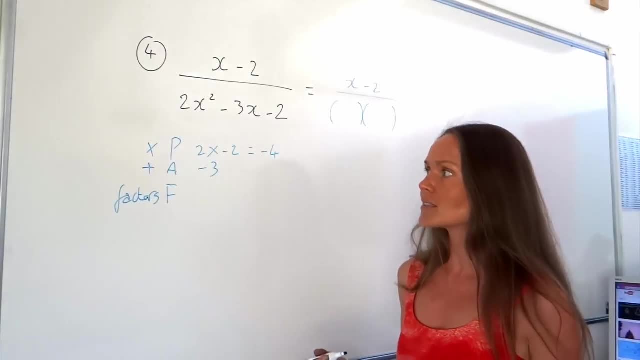 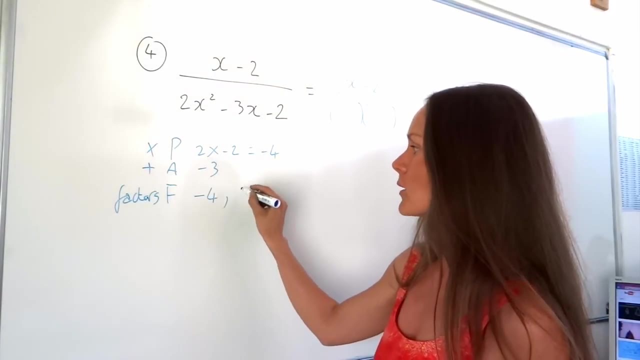 So I'm going to write it out. so I've got x, which is negative 3.. So I need to come up with factors that multiply to give negative 4, and they add to give negative 3.. Well, it must be minus 4 and 1, because when I multiply them I get this, and if I add them I get this. 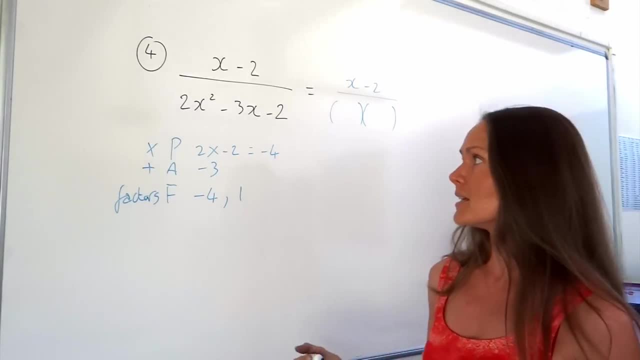 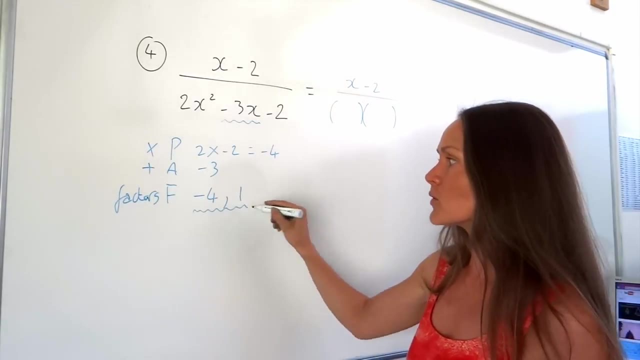 So I've found my factors. So the method with PATH is I have to write out the quadratic again. but when I get to my x term I need to write that in terms of my new factors. So I'm going to write it out. so I've got. 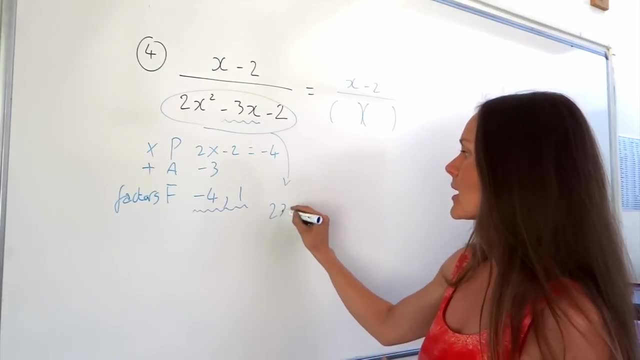 I'll do it in over here. So I've got 2x to the square. just stays the same. Now, instead of this, I've got negative 4x and plus 1x, which is plus x, and then the negative 2 as well. 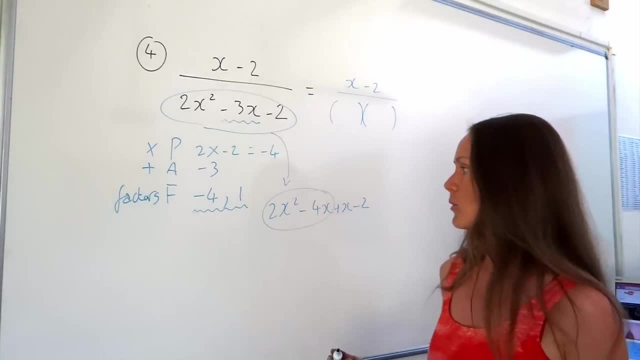 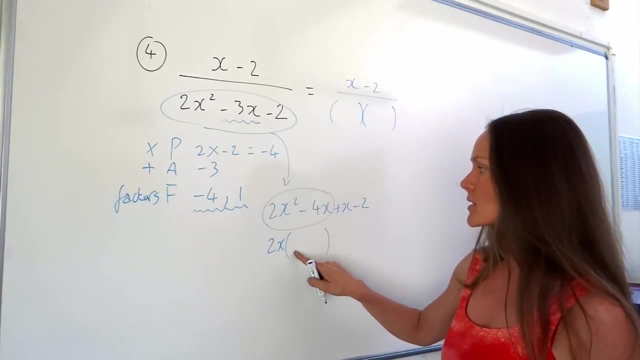 Now I take the first 2 terms and I take out the highest common factor, which is 2x, and I open the brackets. I'm just doing simple, poor factorising. So 2x times something gives me 2x squared, but it must be x. 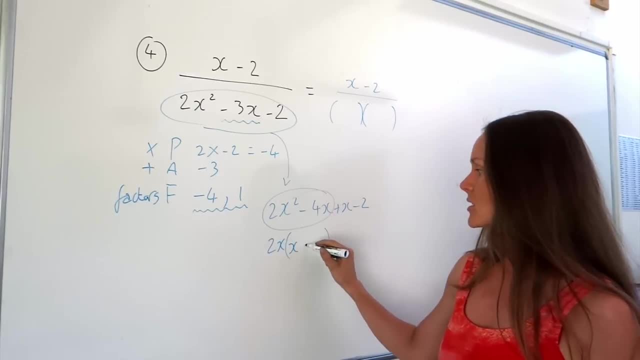 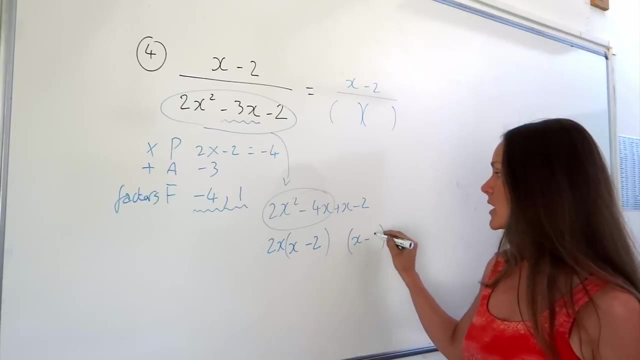 and 2x times something. something gives me negative 4x, which is just negative 2.. Then I just leave a little gap and I write out the same bracket again, Because if I've done it correctly, these brackets should always be the same. And then I decide what goes in front here, so that this is the same as this. 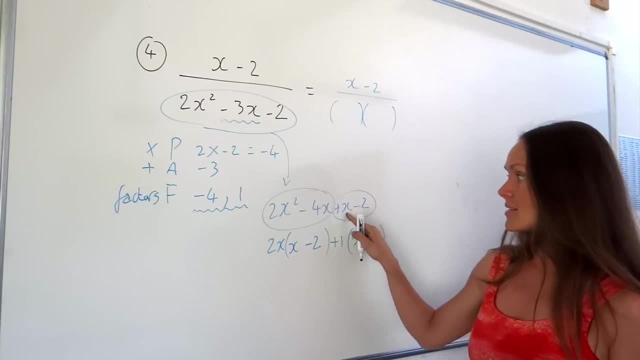 Well, it's just plus 1, because 1 times x is x and 1 times minus 2 is minus 2.. So now that I've got my repeated bracket, I can start to fill in the final factorizing part, The bracket that's. 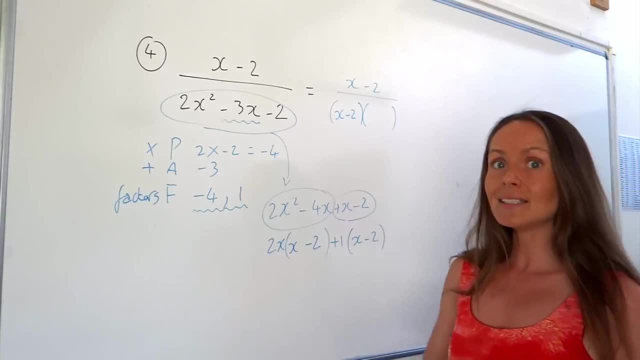 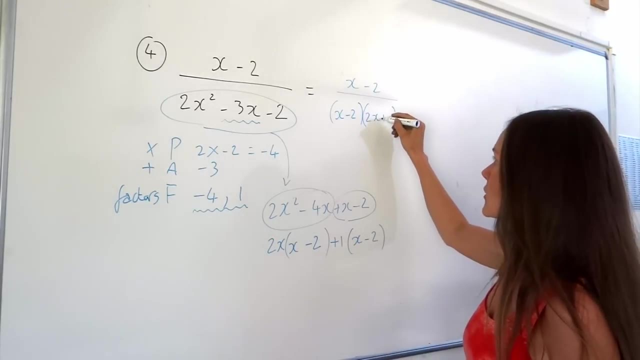 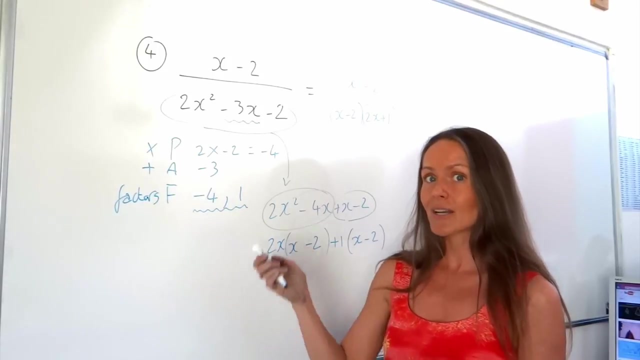 repeated, is one of these, It doesn't matter which one. And in the second bracket are the bits that I left over, So the 2x and the plus 1.. So now I've factorized. So, like I said, if you're not sure about this, I have a whole video explaining path and how to factorize. 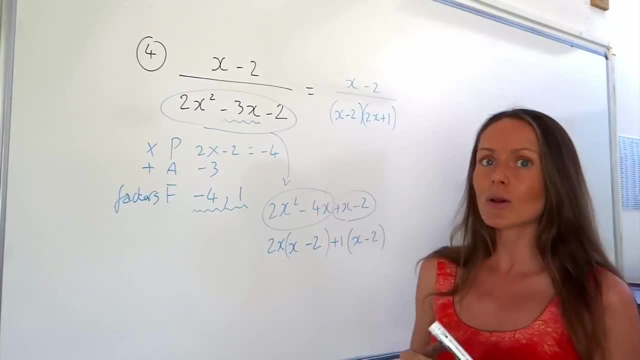 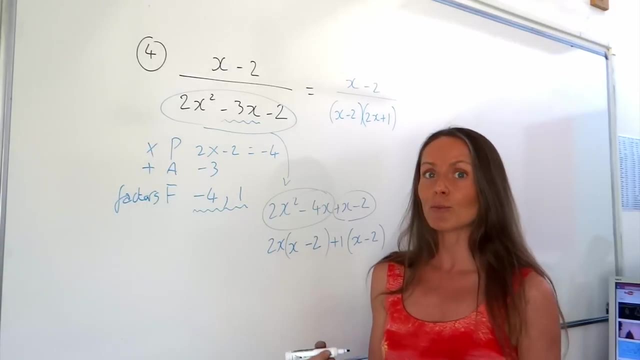 Some people just like to guess And sometimes it won't take you too long to guess. But if you have difficult numbers then it's much better to have a method like path to help you factorize these tricky quadratics when there's a number in front of the x squared. 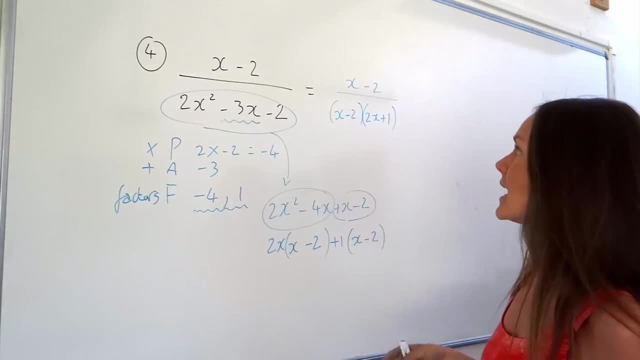 Anyway, back to the simplifying. I've done my factorizing. Now I need to look to see what's common, to see if I can cancel something on the fraction, And I can see x minus 2 on the top and x minus 2 underneath, So I can cancel them out. But you can't just leave it like that, because